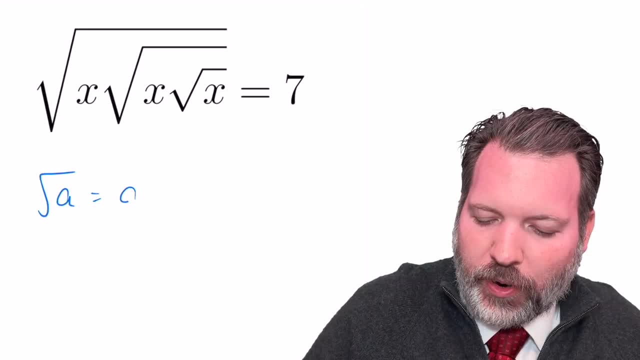 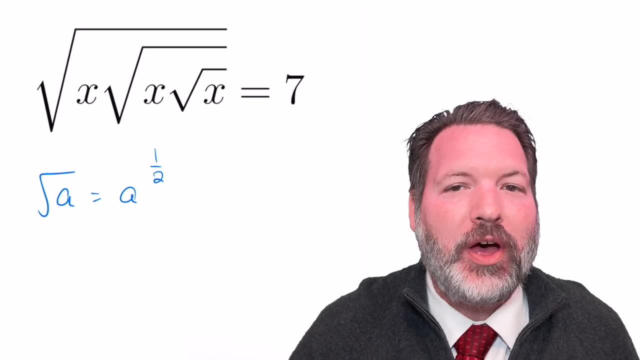 terms of exponents. So to tackle it that way, we have to be aware of this particular equivalence, which is that the square root of something, a, let's say, is the same thing as the half power of a. This is the connection between roots and exponents. Roots are essentially fractional. 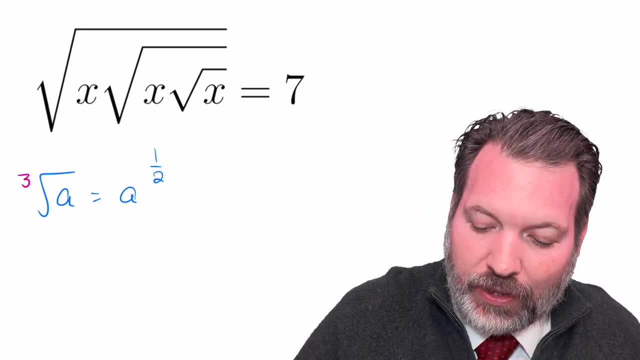 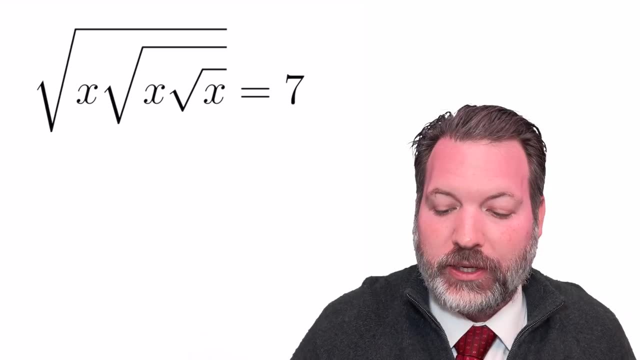 exponents. If this had been a third root, for example, instead, then this wouldn't be the half power of a, It would be the one-third power of a, But it is a square root, and so we're going to use this half power idea to rewrite this expression. This is really going to be something to the one. 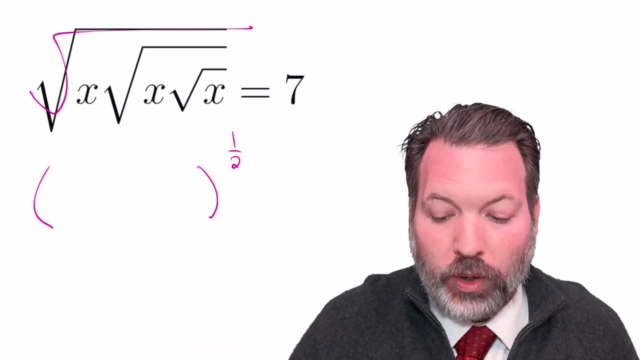 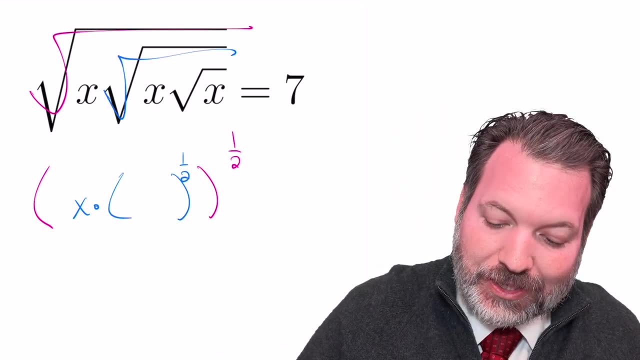 half. That is this big square root on the outside here. What's the something X times another big old square root? That's this second nested square root here. Something else to the half power. What's on the inside of that? something X times one last square. 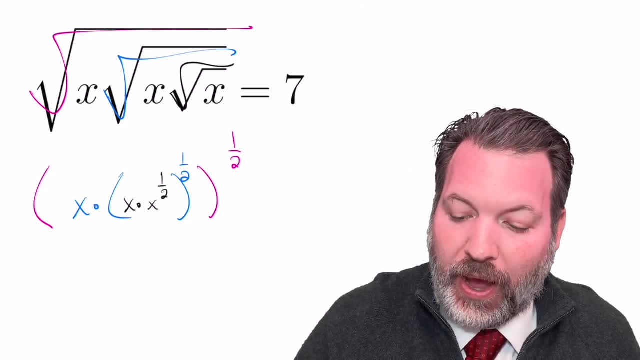 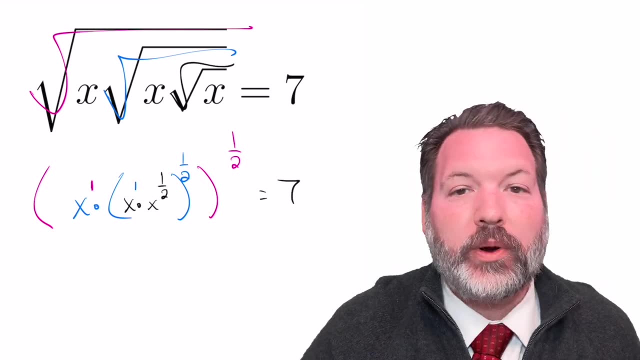 root of x, X times another x to the one half power, And it's all of this that ends up equaling 7.. From here I'm going to plug in some exponents we didn't already place. Everywhere that we have an x, I'm actually going to write an x to the first, and then I'm going to utilize our exponent rules. 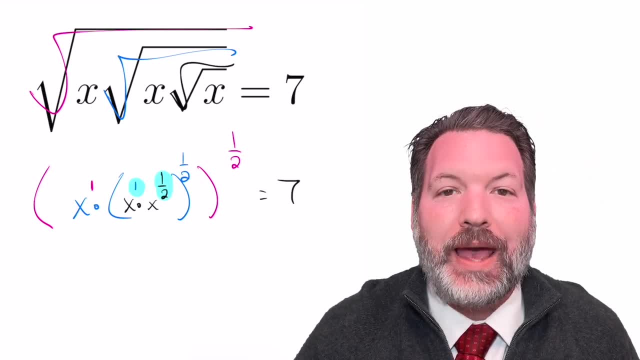 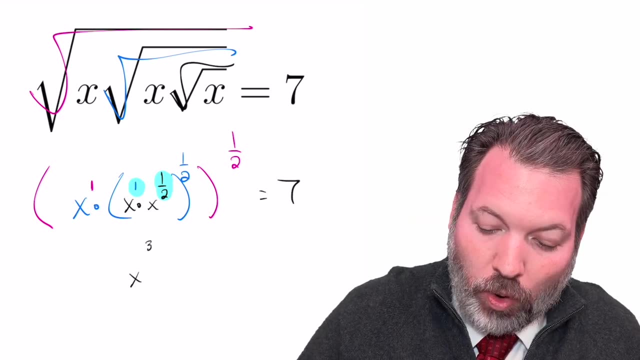 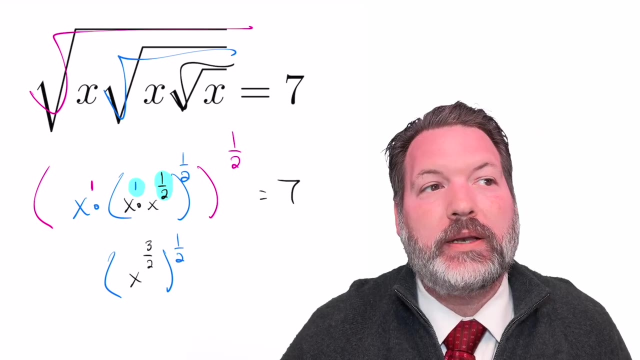 When we are multiplying expressions with exponents, we can add those exponents together, So that inner one times x to the one half is the same thing as x to the one plus one half power, which is x to the three halves power. Now that itself was being raised to the one half power, and I'm going to apply a 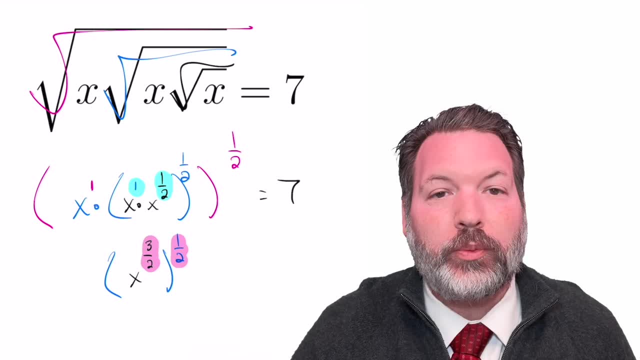 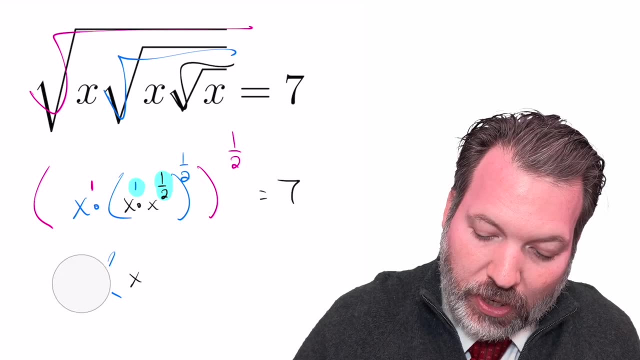 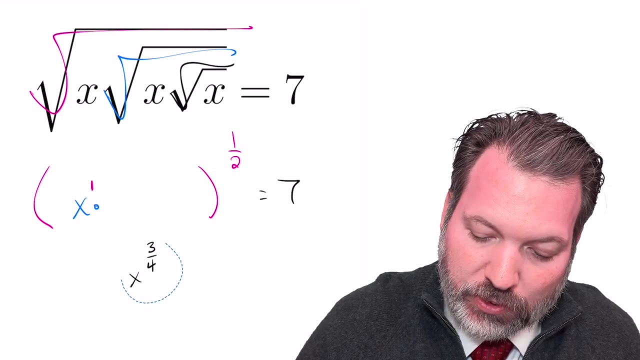 second exponent rule: When we raise a power to another power, we multiply those powers. So x to the three halves to the one half power is the same thing as x to the three fourths power. Three halves times one half is three fourths. Let's do a little housekeeping and go ahead and replace what we've. 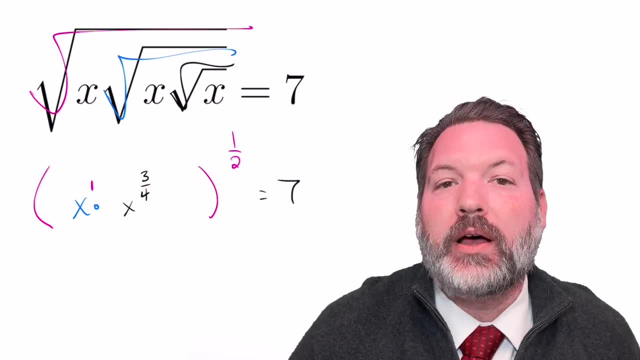 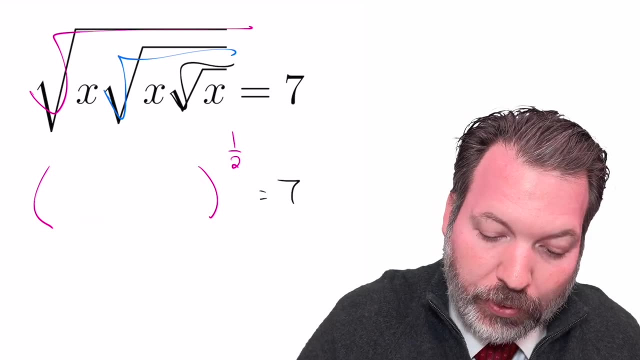 evaluated So far and we can see we have another application of adding exponents here. X to the first times, x to the three fourths is going to be the same thing as x to the one plus three fourths power, That is x to the seven. 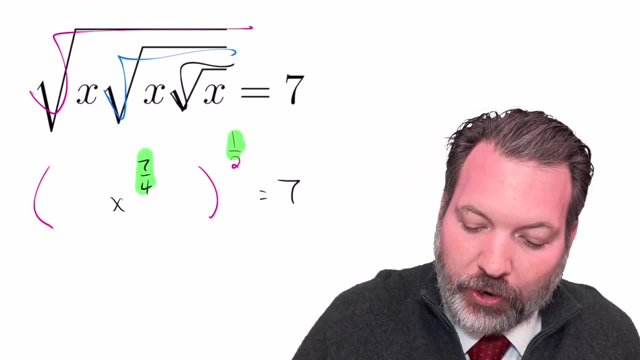 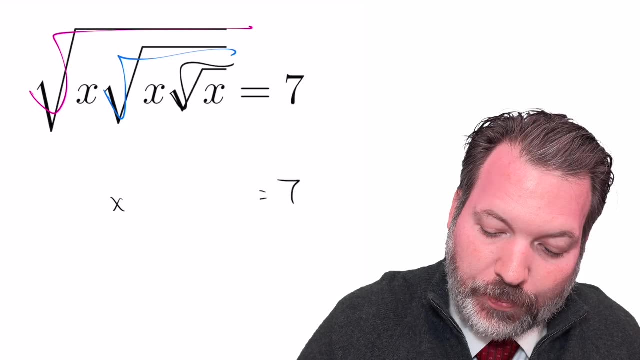 fourths power. And finally, one more time, we've got another exponent to exponent situation. Power to power means multiply, So seven fourths times one half gives us back seven eighths. And this is the scenario we find ourselves in: Some unknown x to the seven eighths power is the same thing as x to the.